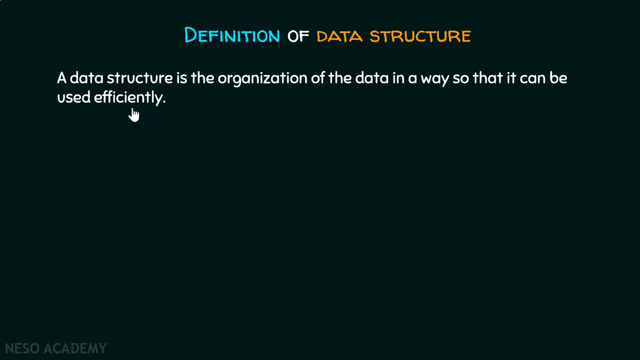 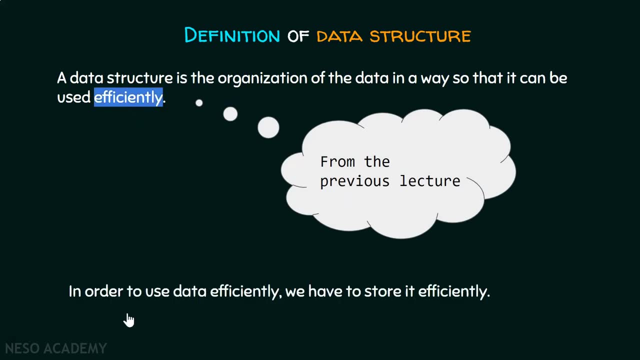 and if we want to use our data, we would be able to use it efficiently. This is the definition I have taken from the previous lecture. right Now, this efficiently term is very important. In order to use data efficiently, we have to store it efficiently. 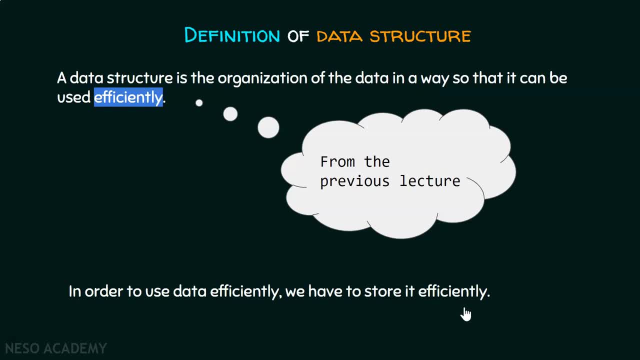 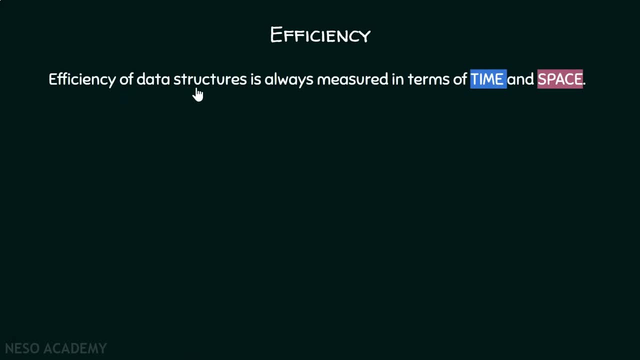 There is no doubt about it: We have to store our data efficiently if we really want to use our data efficiently. Now let's discuss the efficiency in more details. Efficiency of data structures is always measured in terms of time and space. Let me tell you when efficiency comes. 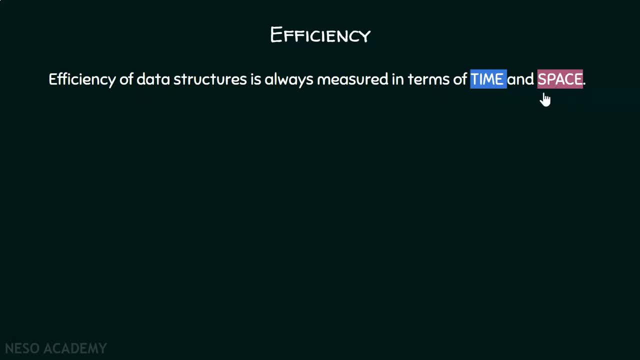 it is always measured in terms of time and space. So what is the picture of an ideal data structure? An ideal data structure could be the one that takes the least possible time for all its operations and consumes the least memory space. Both these things should be less. 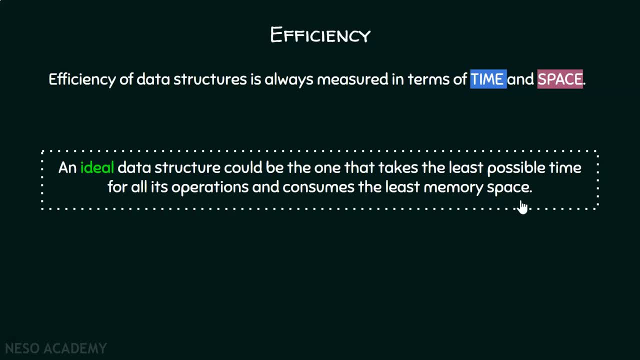 It should take the less amount of time for all its operations and it should consume the least memory space as well. Then I can say a data structure would be an ideal data structure, Isn't that? so Now our focus will be on finding the 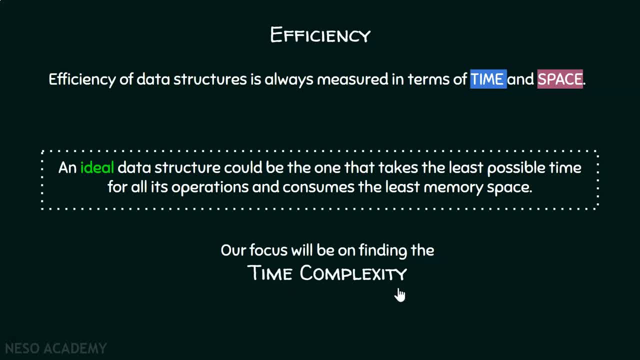 time complexity and not the space complexity. let me tell you, We are not interested in finding the space- that how much space a data structure will consume. We are right now interested in finding the time complexity for easing our task. Okay, So by finding the time complexity. 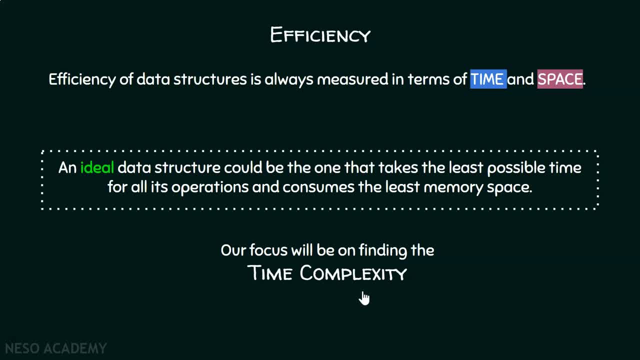 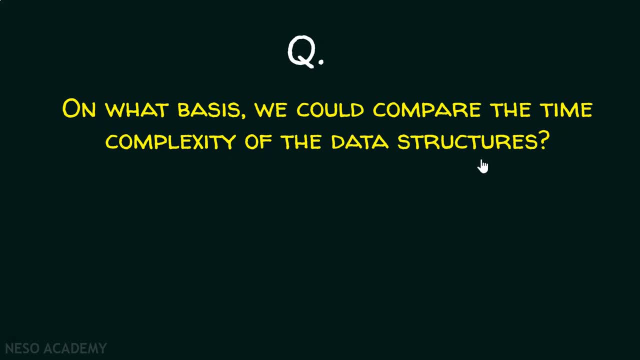 we would be able to guess which data structure would be the best. Okay, Now there is one question: On what basis we could compare the time complexity of the data structures? This is a very important question. let me tell you, We are going to compare the data structures, right? 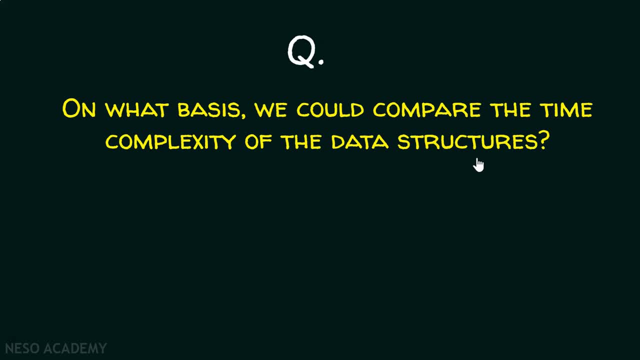 Now how we can compare the time complexity of the data structures. On what basis we will compare it? We will compare the data structures on the basis of operations performed on them. Now let me give you an example and the whole concept will be clear to you. 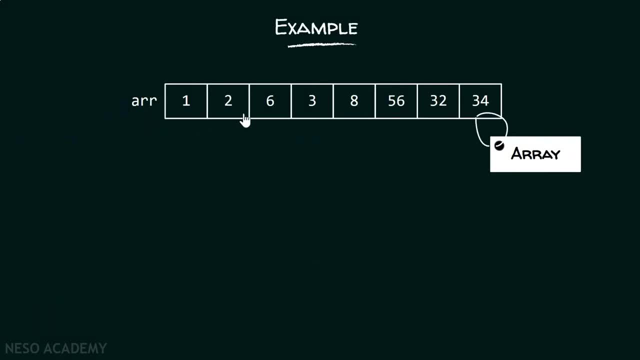 Let's take an example of an array. Okay, Let's say we have these many elements in our array Right now- the size is not defined. But just think of this: that this array is capable of storing hundred elements, and right now we have eight elements in this array. 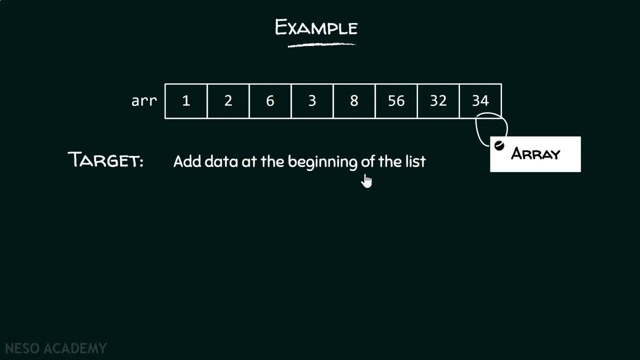 Let's say, our target is to add data at the beginning of the list. This operation we want to perform on this array. Array is a data structure. We want to perform this operation, that is, adding data at the beginning of the list, And I want to know that, how much time it will take. 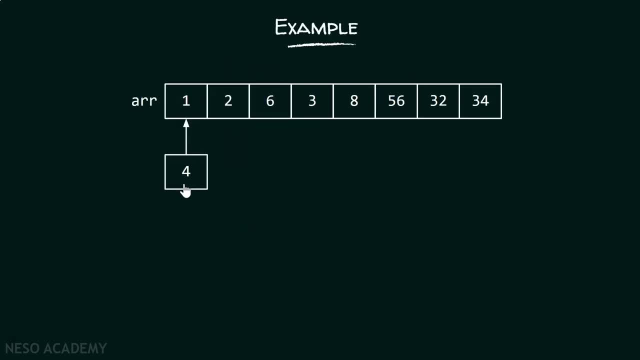 Let's study this properly. Let's say, we want to add this particular element at the beginning of the list. Now, obviously, this element is trying to reach this particular place slowly. There is already an element at the beginning of the list, Isn't that so? 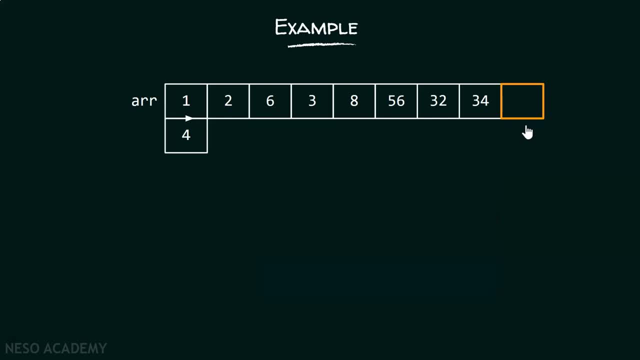 There must be an empty slot available in the array. As I have already told you, my array is capable of storing hundred elements, So obviously there is an empty slot over here. Now, what we will do is we will shift all the elements towards right. 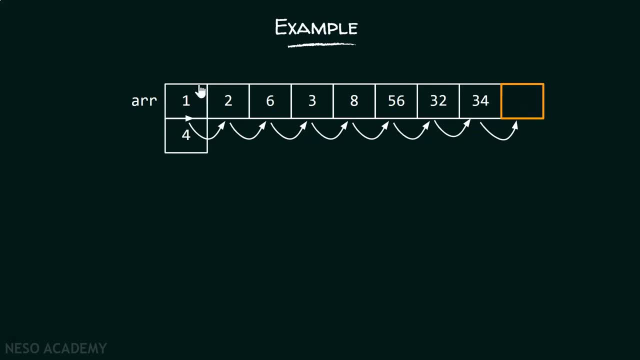 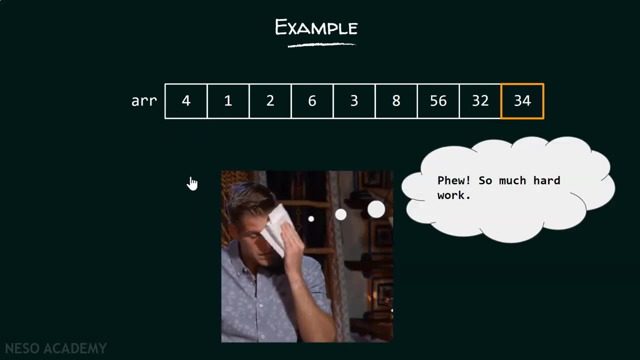 These elements. we will shift towards right so that there should be an empty slot over here. Then we can easily add our element at the beginning of the list. Oh my god, there is so much hard work, right, If we want to add an element at the beginning of the list. 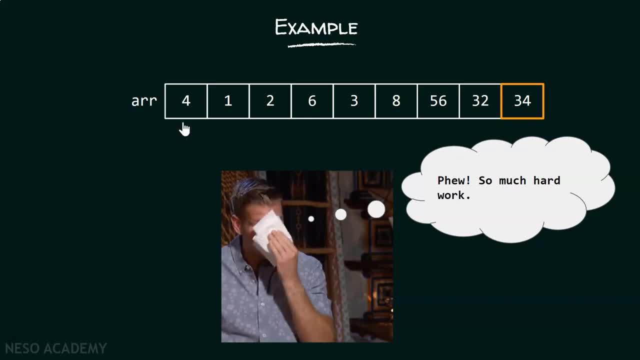 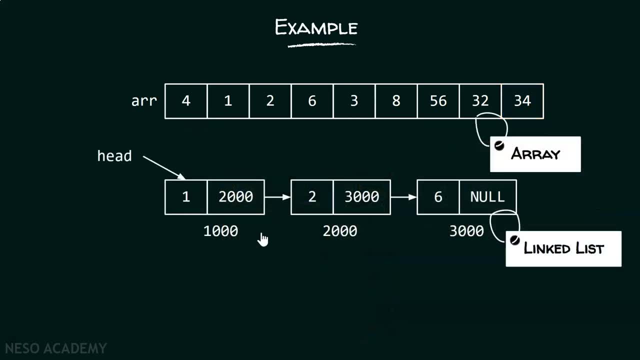 and that to an array. it would be a very difficult task. We have to shift our elements towards right and then we can add our element. Let's take another type of a data structure, that is linked list. Linked list is nothing but sequence of nodes connected with each other. 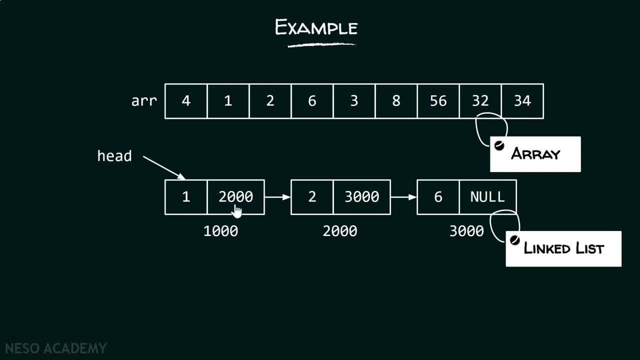 Here we have this node, which contains some data, and it also contains the address of the next node. Okay, Now, the difference is that an array is stored in a contiguous fashion, That is, obviously, if the address of this particular element is 1000, then the address of the next element. 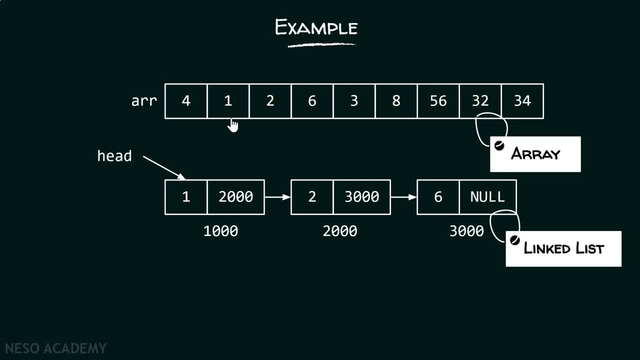 will be 1004, if I am assuming that size of integer is 4 bytes. right, But here it is not important. It might be possible that the address of the one node is 1000 and the address of the next node is 2000.. 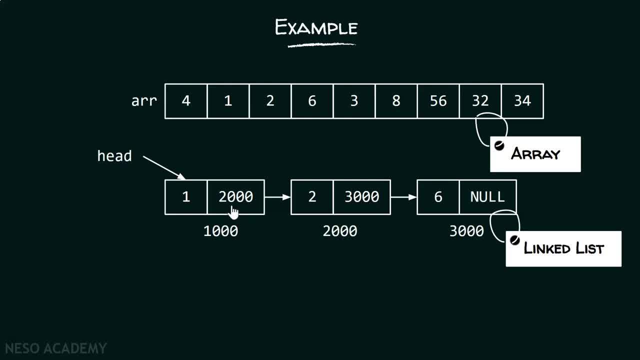 It could be any address. Let's store the address of the next particular node so that it can be linked to the next node. So this is what a linked list is all about, And obviously there is a head pointer which is pointing to the first element of the list. 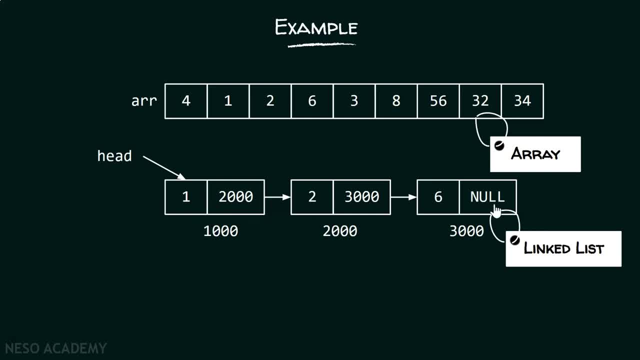 so that we can reach the first element and then, after that, we can reach the other elements as well. This is what a linked list is Okay. Now let's say we want to add this particular data in the beginning of the list. Now, how do we do that? 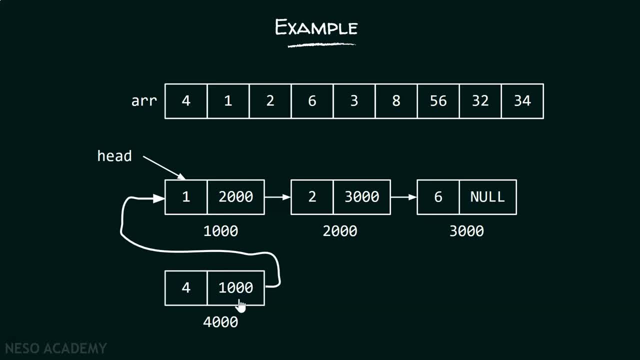 We definitely have to store the address of this particular node over here, right? So let's replace this by 1000.. Using this address, it will point to this particular location. Now this node is linked to this node. After that, we just change the head pointer.